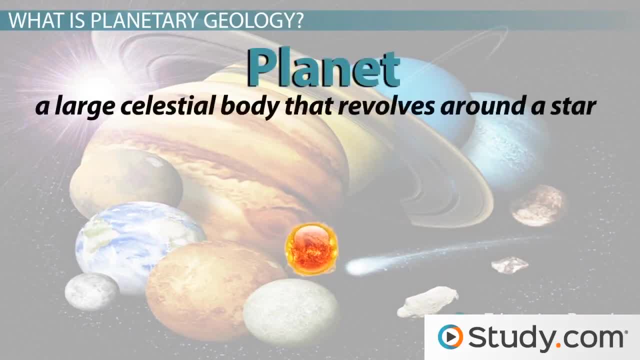 between these celestial bodies. A planet is a large celestial body that revolves around a large celestial body. A large celestial body is a large celestial body that revolves around a large celestial body. A large celestial body is a large celestial body that revolves around a star. A moon is a celestial body. 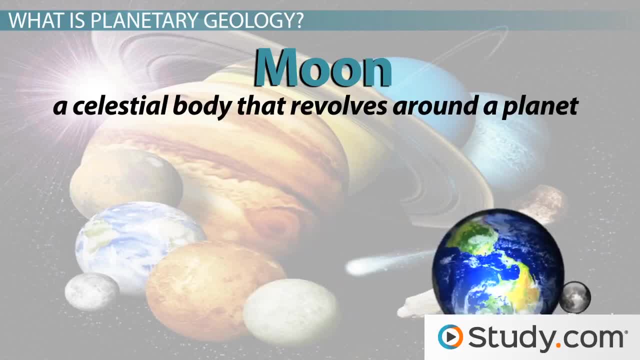 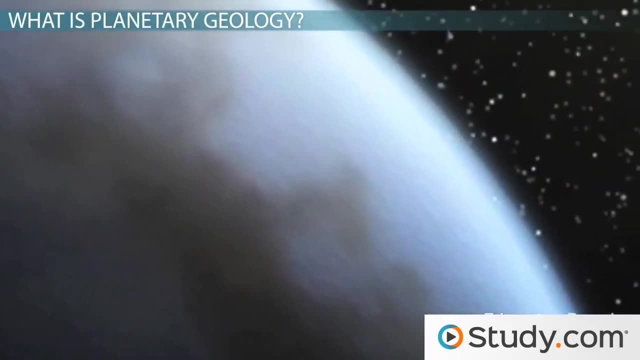 that revolves around a planet. Our planet Earth has only one moon, but other planets have multiple moons that orbit around them Besides Earth. Earth's moon is the only other celestial body that humans have set foot on. Planets and moons are the larger celestial. 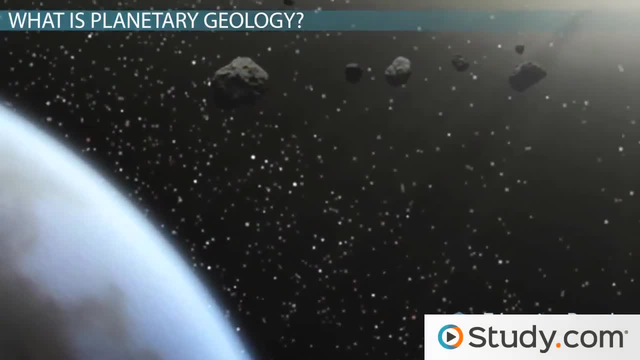 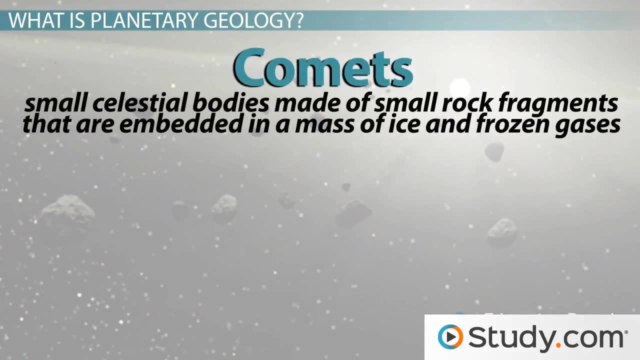 bodies found in the solar system. Smaller celestial bodies include comets and asteroids. Comets are small celestial bodies made of small rock fragments that are embedded in a mass of ice and frozen gases. Most comets orbit the sun and take several years to complete. 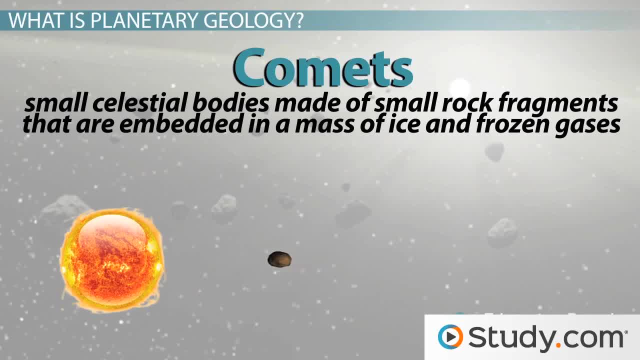 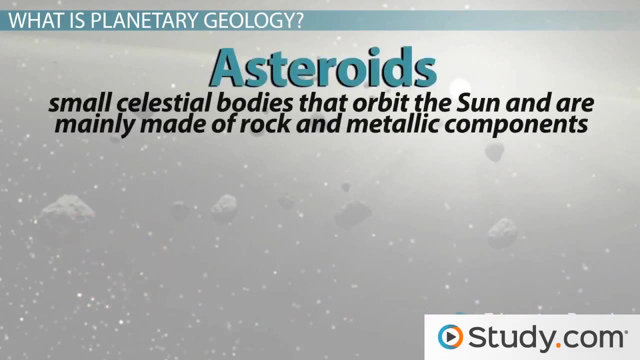 the journey. There are also comets that have journeys that take up to 3 million years. When a comet gets close to the sun, it begins to evaporate, which releases a stream of molecules behind the comet that forms the characteristic tail we see from Earth. Asteroids are small. 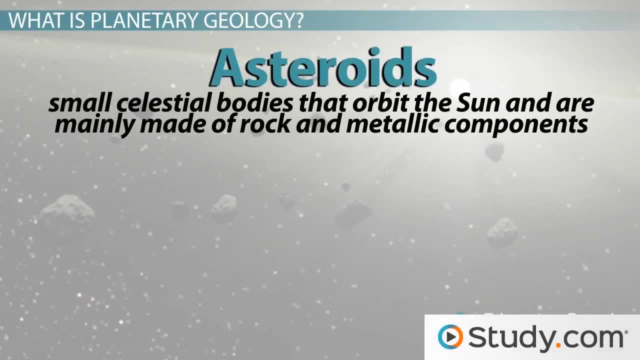 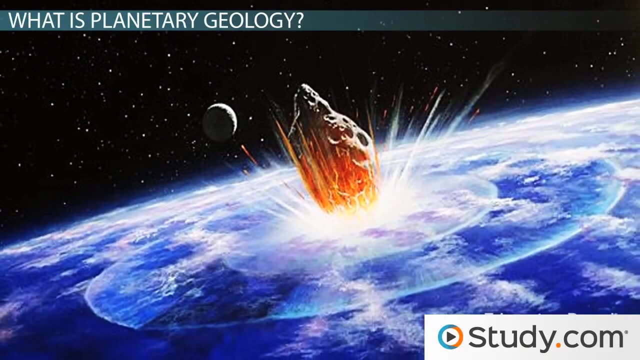 celestial bodies that orbit the sun and are mainly made of rock and metallic components. If asteroids collide with each other, they can be thrown off their normal orbits and travel in any direction. This can result in an asteroid colliding with another celestial body, most frequently planets. Now that we know what planetary geology is and what celestial 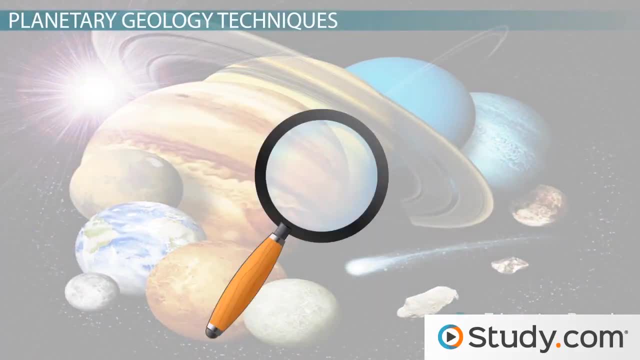 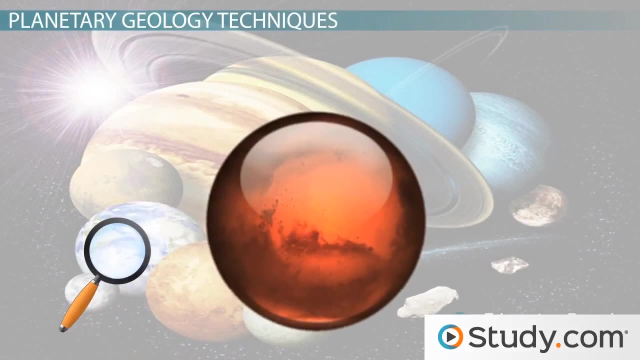 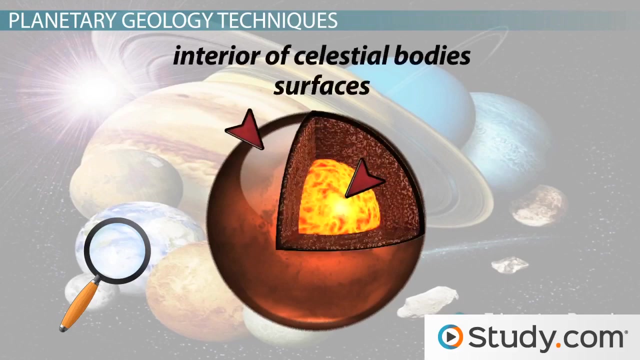 bodies are. let's examine what exactly planetary geologists study, why they study it and how they study it. Planetary geologists study the solid matter that makes up celestial bodies. This means that they study the interior of celestial bodies as well as the surfaces There are. 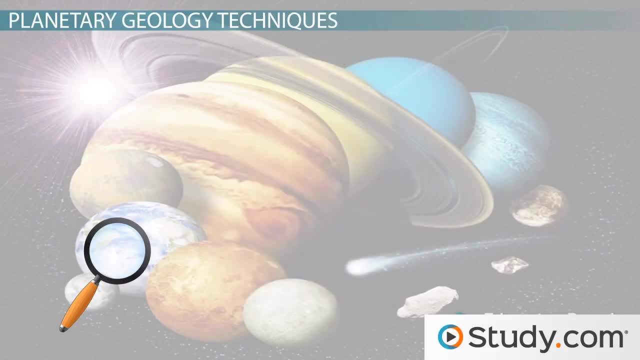 many reasons why planetary geologists study celestial bodies. One main reason is just to learn more about the world around us. We are curious and want to know what else is out there beyond Earth. Planetary geologists also study the composition of celestial bodies. They study the composition. 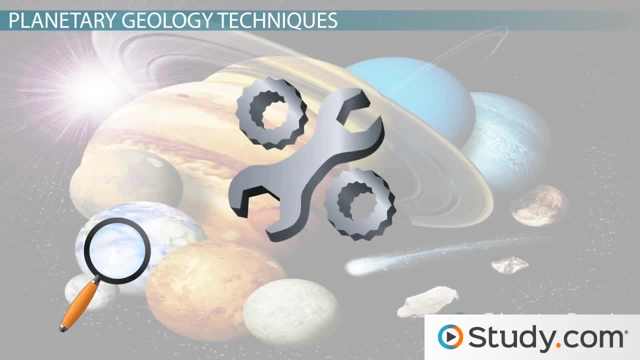 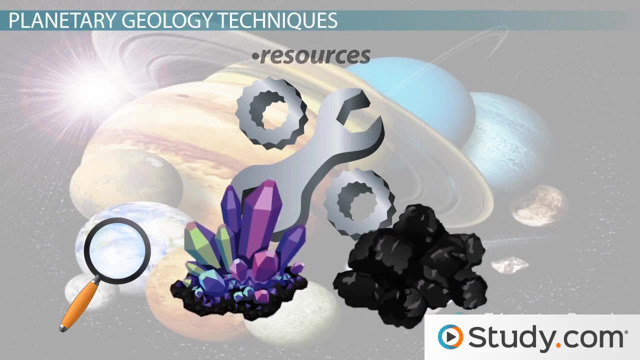 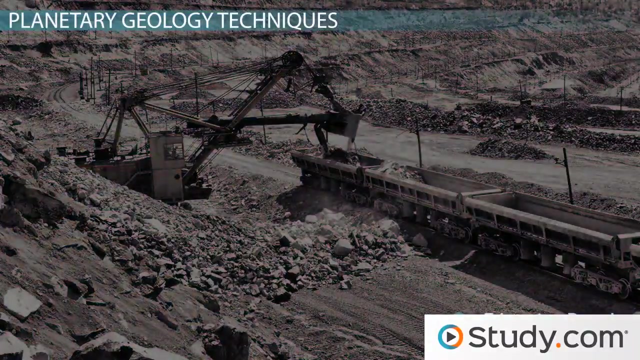 of celestial bodies to determine how they were formed and if there are any natural resources such as minerals or energy sources available within the celestial body. As humans diminish the natural resources on Earth, some people believe that other celestial bodies might provide necessary resources. Another reason: planetary geologists study celestial bodies. 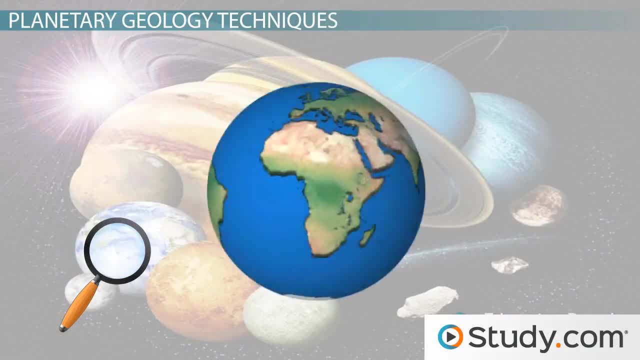 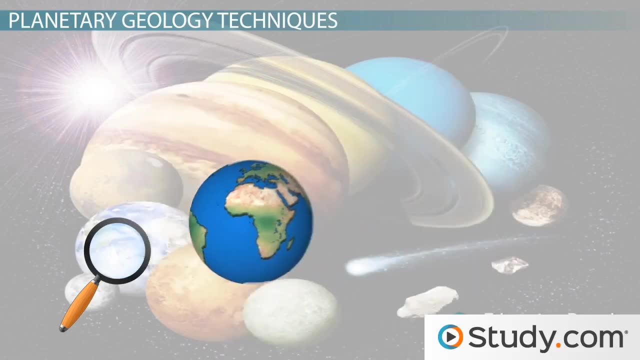 is to determine if there is life on these objects. Geologists that study Earth have an advantage because they can examine celestial bodies. They can determine if there is life on these objects. Geologists that study Earth have an advantage because they can examine it with their own hands. Planetary geologists face the challenge of trying to study something. 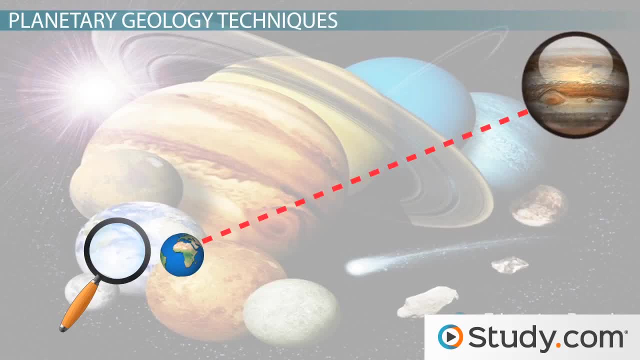 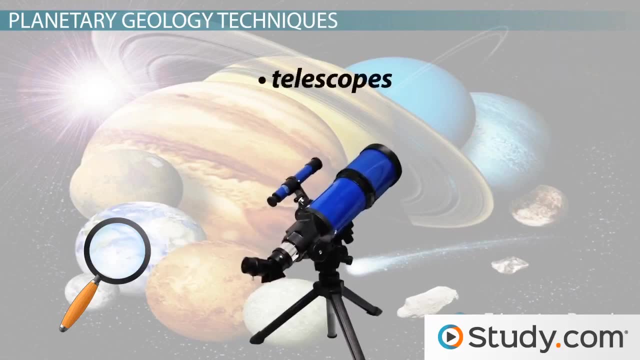 that is very far away and cannot be reached by human hands. Planetary geologists use a variety of techniques to overcome this challenge. One technique is the use of telescopes. Telescopes allow scientists to get a close-up look at the surfaces of celestial bodies. Scientists 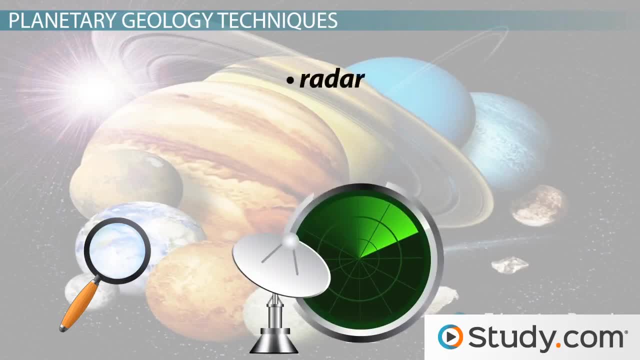 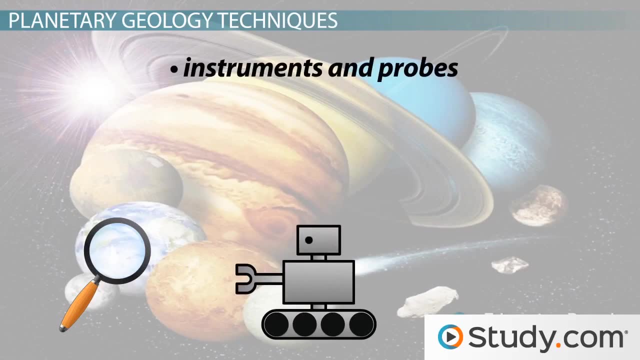 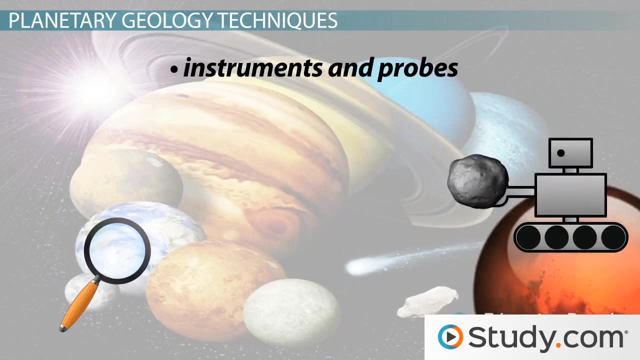 also use radar to study the topographic features and texture of the surfaces of celestial bodies. To investigate the interior of celestial bodies, scientists rely on instruments and probes. This equipment can be launched to celestial bodies from spacecraft and remotely controlled. These instruments can collect rock samples and make close-up observations of the surface. 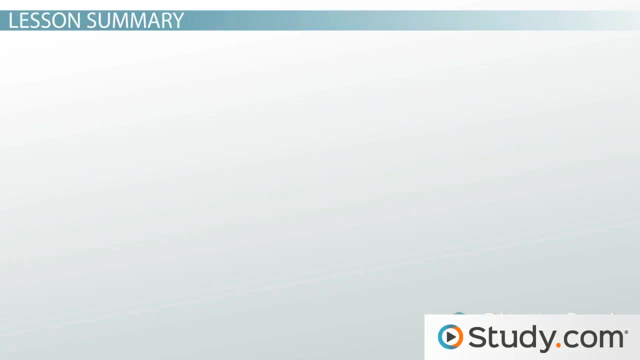 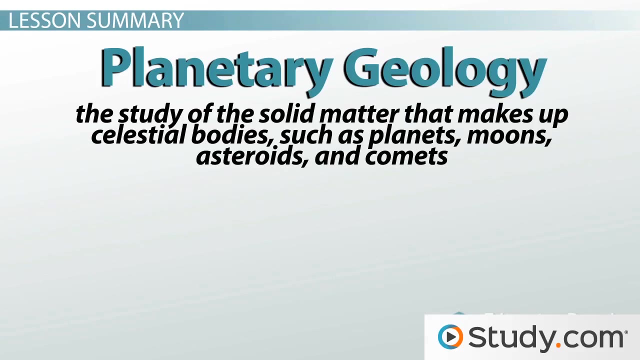 of celestial bodies. Now let's review planetary geology, which is the study of the solid matter that makes up celestial bodies such as planets, moons, asteroids and planets. But before going into the details, let's start by looking at planetary geology in今日's video. 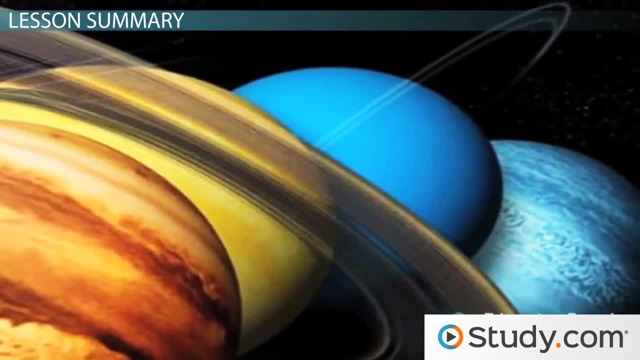 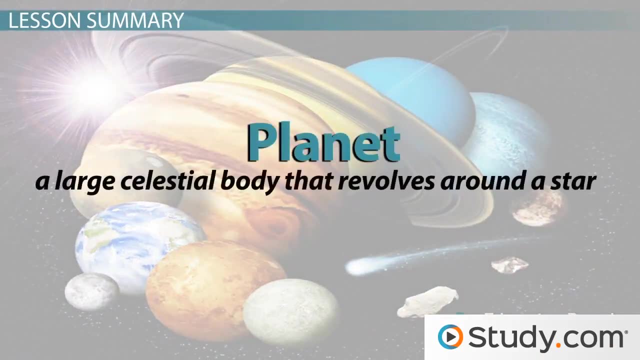 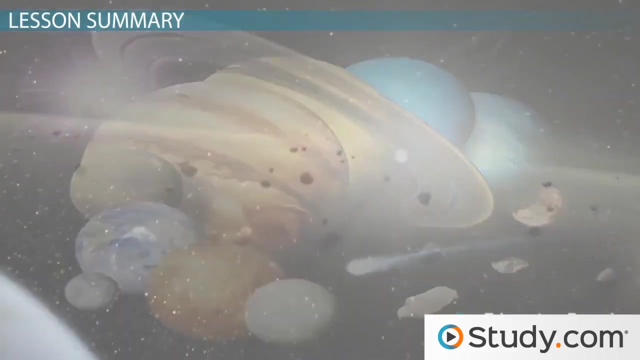 and comets. There are several different types of celestial bodies that are studied, including planets, moons, comets and asteroids. A planet is a large celestial body that revolves around a sun, And a moon is a celestial body that revolves around a planet. 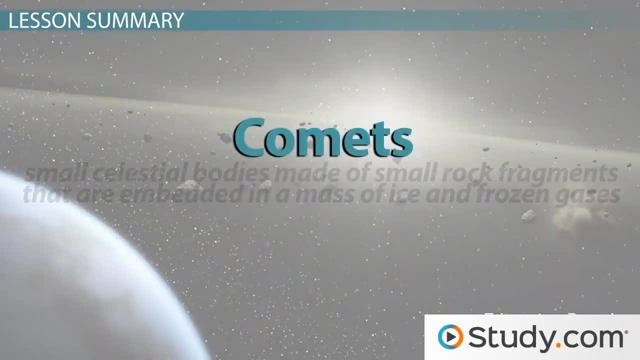 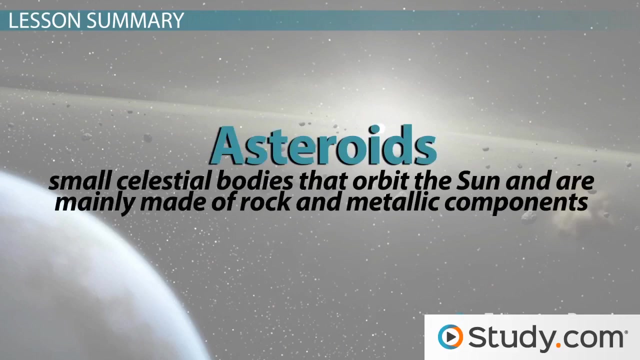 Comets and asteroids are smaller than planets and moons. Comets are small celestial bodies made of small rock fragments that are embedded in a mass of ice and frozen gases, And asteroids are small celestial bodies that orbit the sun and are made of mainly rock and metallic components. 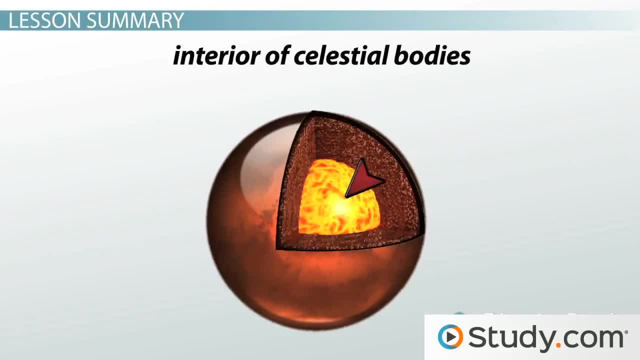 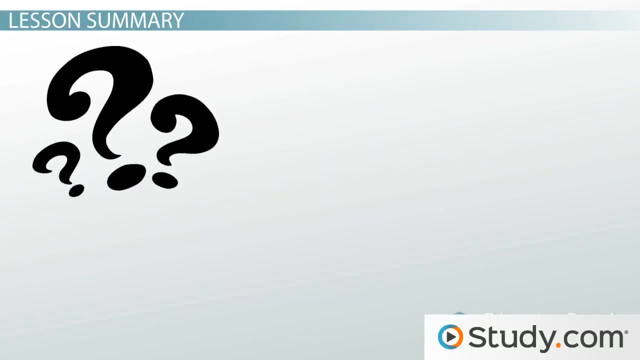 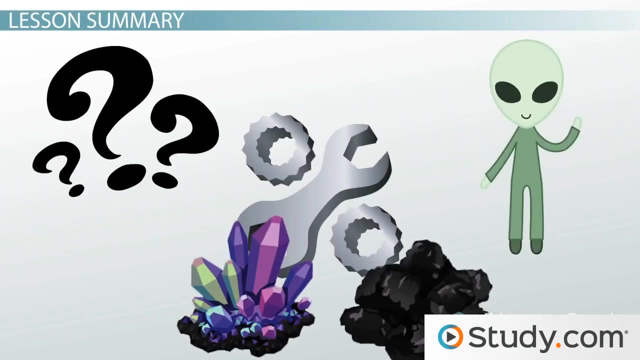 Planetary geologists study the interior of celestial bodies and also the surfaces. They study celestial bodies for many reasons. Some of these reasons include general curiosity, the search for natural resources to determine how celestial bodies were formed and to determine if life exists beyond Earth.